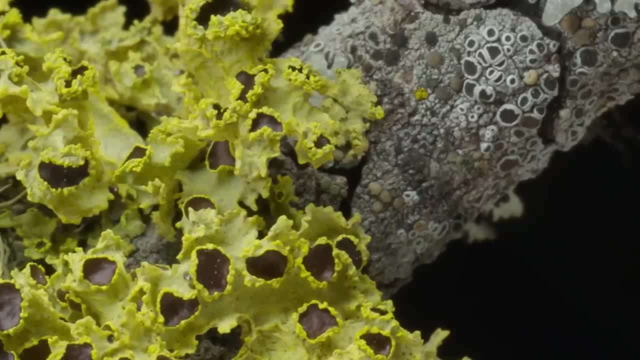 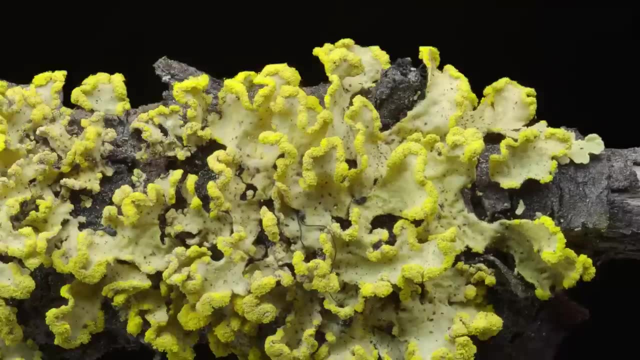 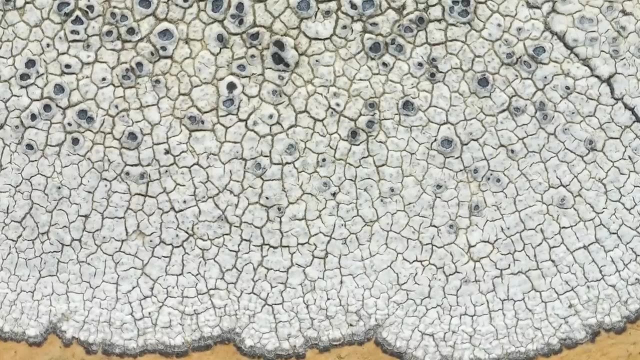 a lichen was assumed to be a union between a single species of fungus and a species of green algae, But when they come together they form this unique structure. unlike the two individuals. The algae photosynthesizes and the fungus produces the structure and those two come. 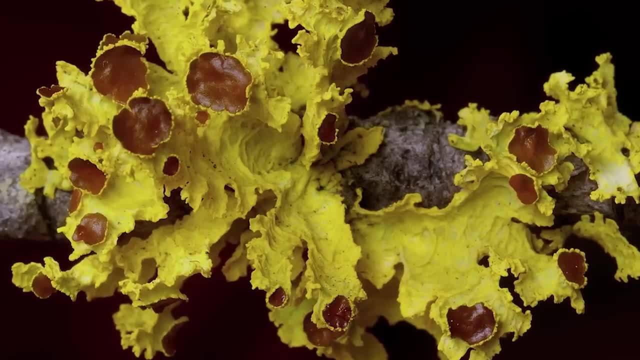 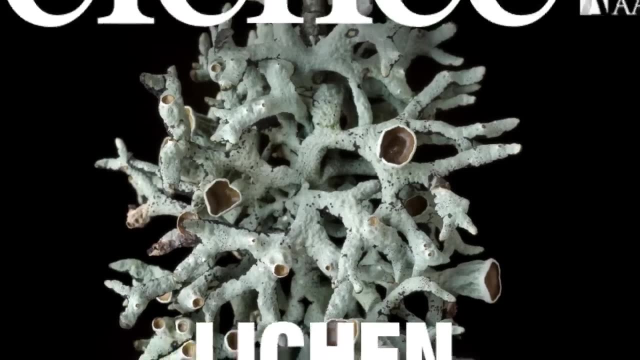 together and they live in places where the individual parts alone couldn't, And that's what we thought of lichens for the last 150 years. The study was accepted in Science Magazine and Toby, the main author on the paper, approached me and asked if I would do a photo for the cover. 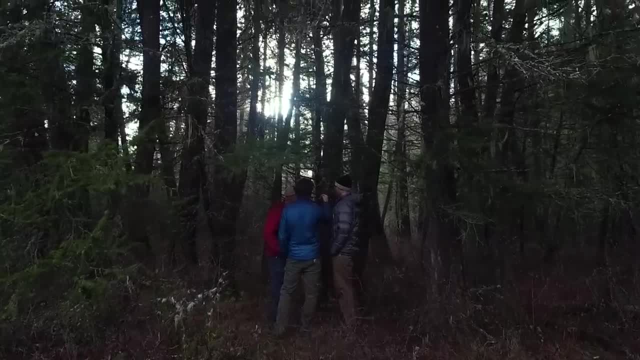 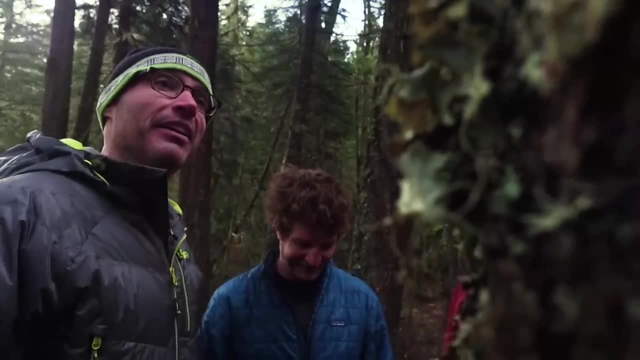 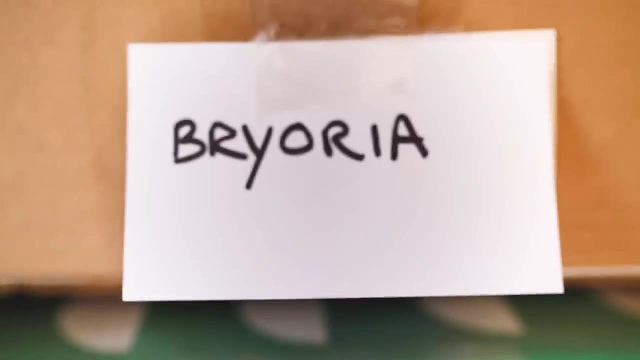 Ultimately, I just told him I am in between this individual and lichen. This person, Toby Sprabila, walks in And I don't know what he said: Hi, I'm Toby, I work on lichens, Please sit down. And So Toby brought me this problem is he's. 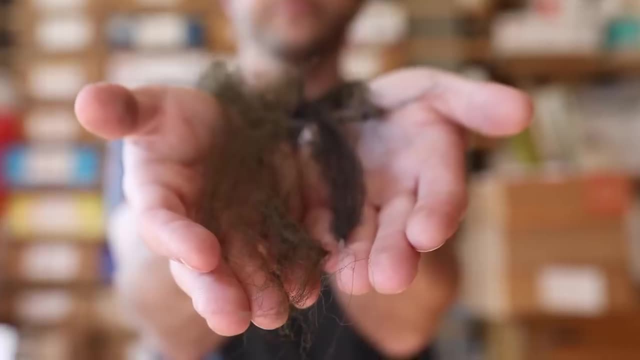 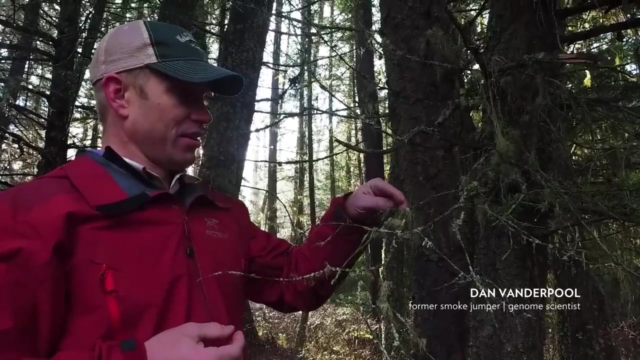 had these two lichens that were clearly different. demise between flying those from the surface of the level and hitting them with value for them, wr Iowa's red Sbornstein" chap movement of the earth. they were exactly the same. Native Americans used the edible horsehair. 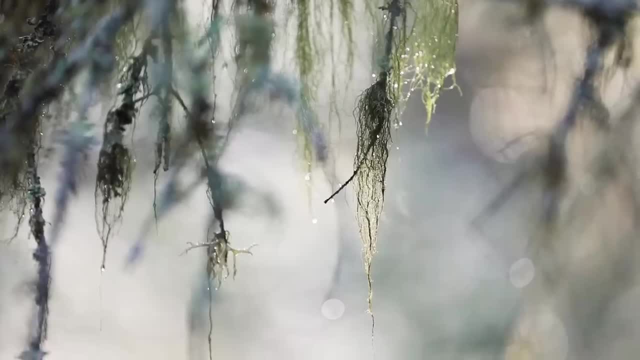 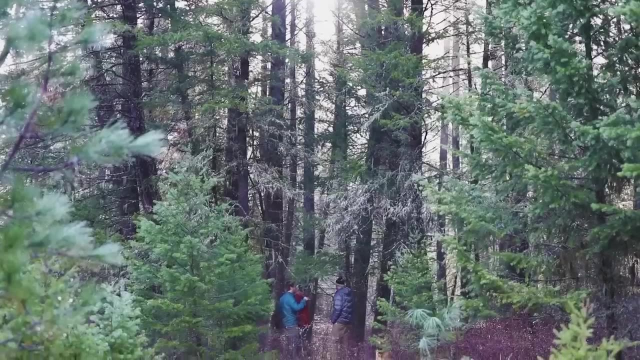 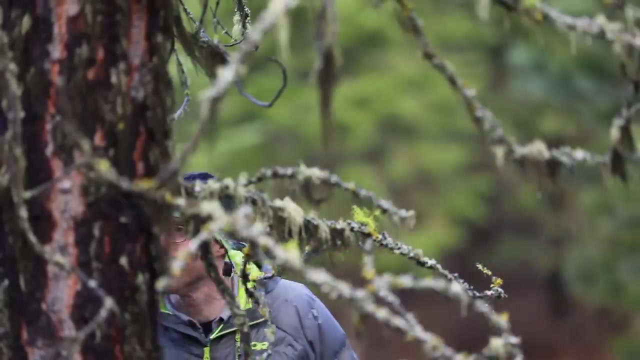 lichen that brown stuff hanging from trees and essentially make little cliff bars. They knew that one was yellow because it contained an acid called volcanic acid and they knew that that was toxic. You're sort of left with this problem of they are different but we don't see it. So what is it? That's the 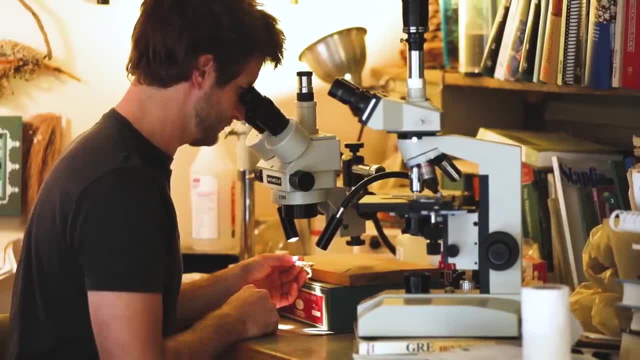 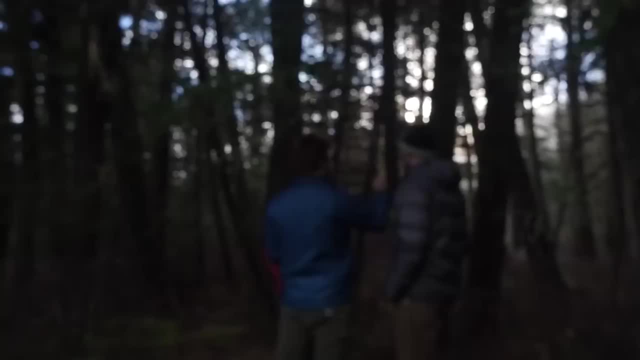 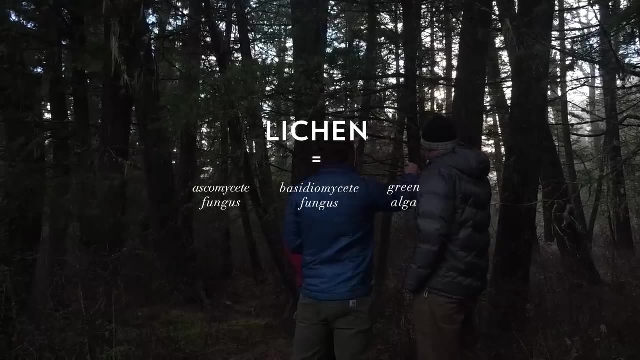 problem. We were stuck thinking about this idea of one fungus, one algae, which is how it's taught in textbook. It was totally wrong. it was absolutely wrong. Well, what we found was that there was a third player, a separate, distantly related fungi that was an integral part of the symbiosis. It took us realizing that. 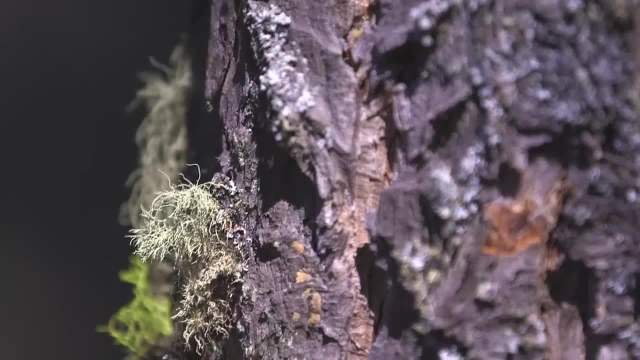 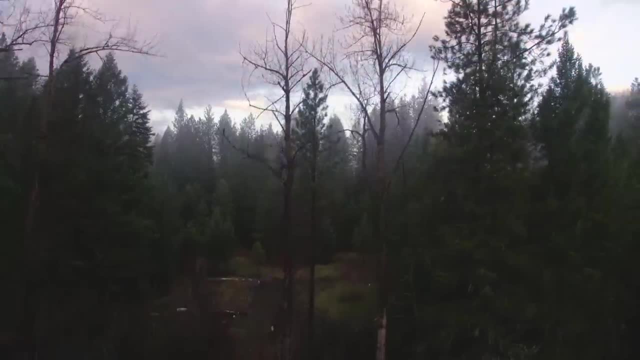 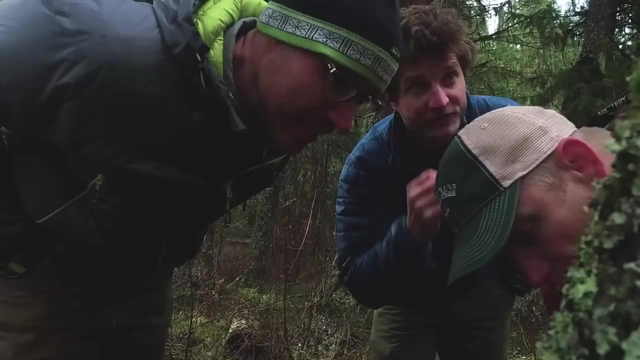 to change how we thought about the symbiosis in general. We looked for, We looked for, We looked for for this additional partner on six different continents And in every case we were finding it. It started as a small project in Montana between a couple of people with different backgrounds.